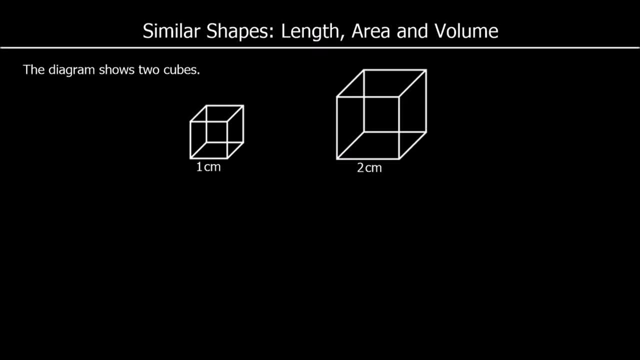 We can say that two shapes are similar if there's been a uniform enlargement, so all of the lengths of a shape have been multiplied by the same scale factor. Here I've got two cubes, and cubes are always similar shapes because if you didn't multiply them by the 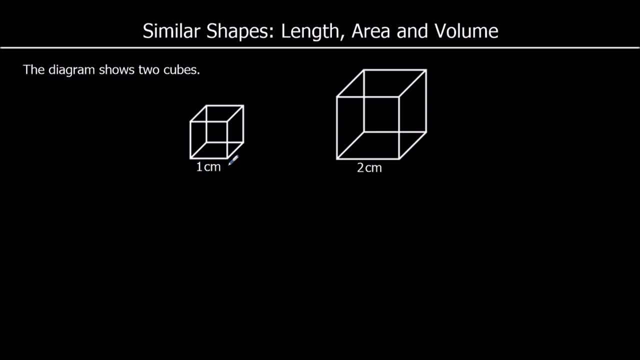 same scale factor. so if you multiplied the width by 5, but the height by 2,, it would no longer be a cube. So let's look at these two cubes. So we've got a 1 cm cube. so it's. 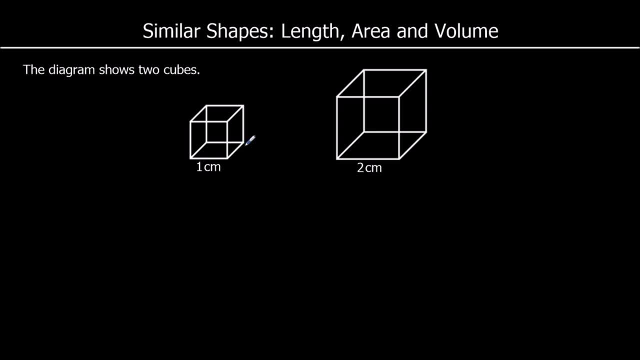 got a width of 1,, a height of 1, and a depth of 1.. And my 2 cm cube has got a width of 2,, a height of 2, and a depth of 2.. So the length scale factor. 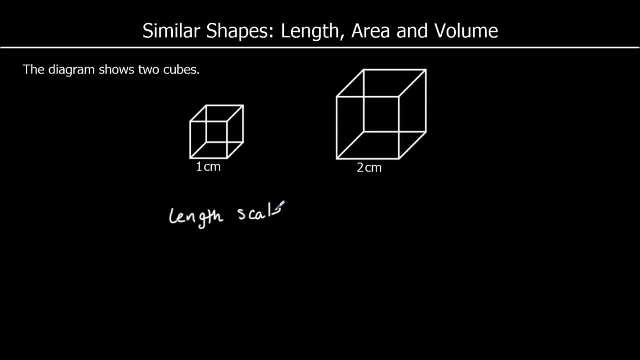 is 2.. We can see it is 2.. To get from 1 to 2, you multiply by 2.. How about the scale factor for area? Is it times 2?? So let's look at a cross section. so the square on the front. 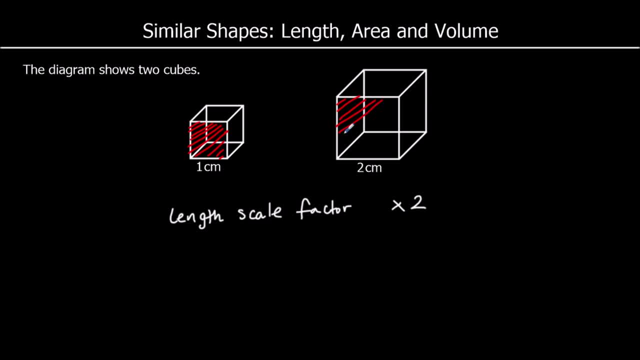 of the shape square on the front of both of these shapes. So for the 1 cm cube you have a height of 1 cm, a width of 1 cm, so its area is 1 times 1, which is 1 cm squared. 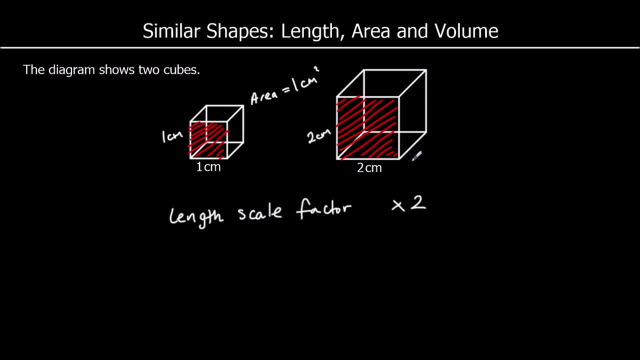 For the 2 cm cube. it's got a width of 2 and a height of 2, so it's got an area of 2 times 2, which is 4 cm squared. So the area scale factor is 2,. 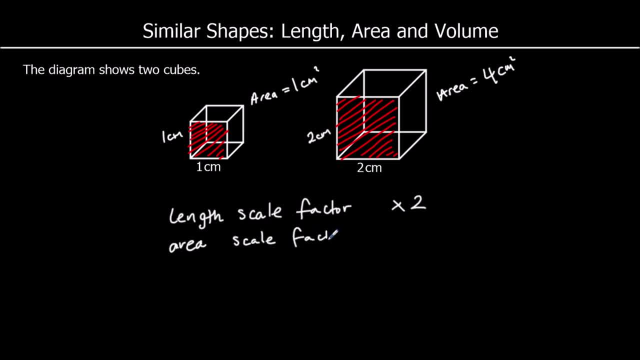 isn't times 2, it's actually times 4, or I'm going to write that as times 2, squared in brackets, times 4.. And how about the volume? So the volume of my 1 cm cube is 1 times 1. 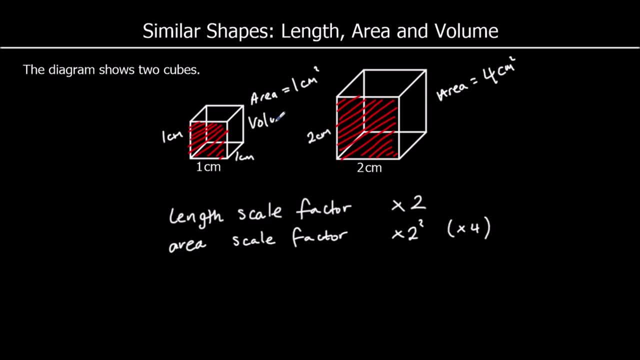 times 1.. 1 times 1 times 1 is 1, so it's got a volume of 1 cm cubed. For the 2 cm cube, it's got a volume of 2 times 2 times 2, which is 8 cm. 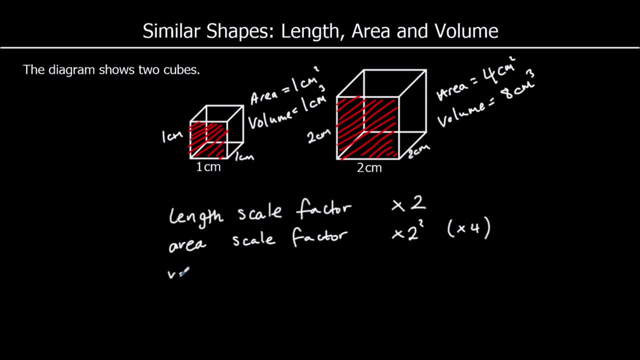 cubed. So the volume scale factor is times 2 cubed or times 8.. And this is the power pattern that we're going to see when we're using area and volume scale factors. So the area scale factor is length scale factor squared and the volume scale factor is going to be: 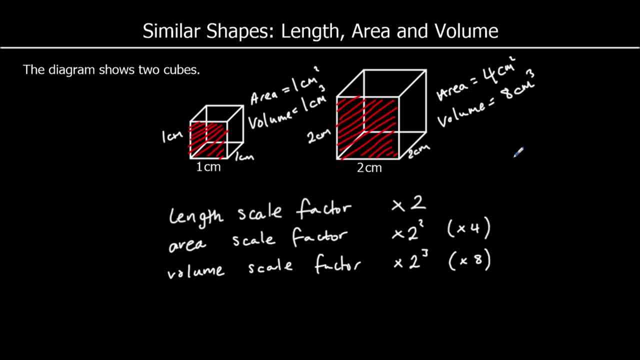 length scale factor cubed. So if we had a length scale factor of 5, so if we had a length scale factor of 5. Our area scale factor will be times 5 squared, or times 25, and our volume scale factor will be times 5 cubed, or times 125.. Okay, let's look at an example. The diagram shows: 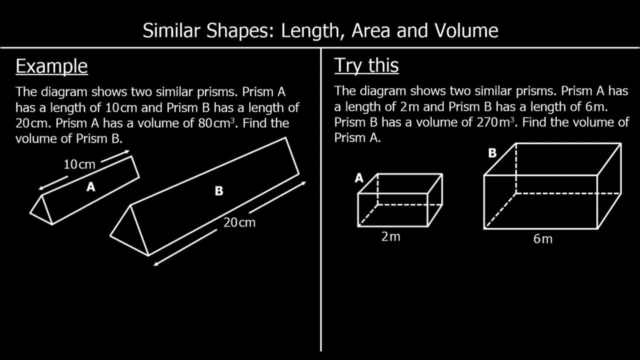 two similar prisms. Prism A, our smaller prism, has a length of 10 centimetres, and prism B, the larger one, has a length of 20 centimetres. Prism A has a volume of 80 centimetres cubed. 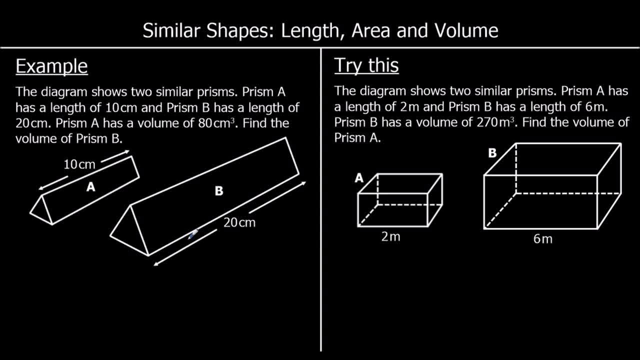 Find the volume of prism B, So we can find our scale factor for length first. So what do we do to get from little shape to big shape? To get from 10 to 20.. So scale factor for length is multiplied by 2.. 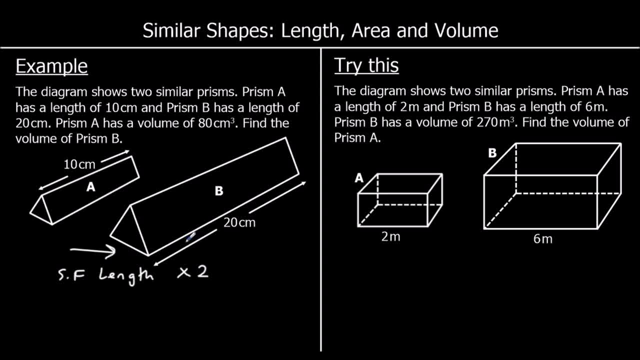 So to go from little shape to big shape, we multiply by 2.. For volume we're going to have scale factor cubed. So for area we've got scale factor squared For volume scale factor cubed. So 2 cubed is 8.. So the volume scale factor is going to be times by 8.. So little shape has a 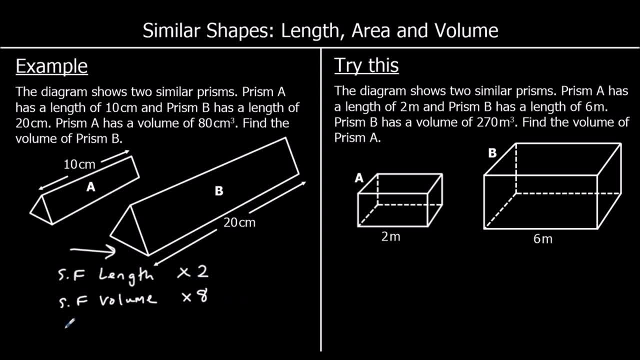 volume. The scale factor is times by 8 for volume. So we've got 80 times 8.. 8 eights are 64. So 88 is 640 and it's in centimetres cubed. So that is the volume of prism B. Okay, one for you to try So. 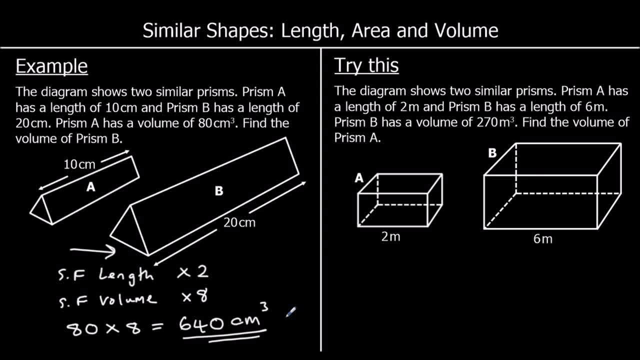 pause the video and give it a go. So again we've got two similar prisms. We've got prism A, our small one, with a length of 2, and prism B with a length of 6.. This time we're given prism B's volume, So 217 metres cubed. Find the volume of 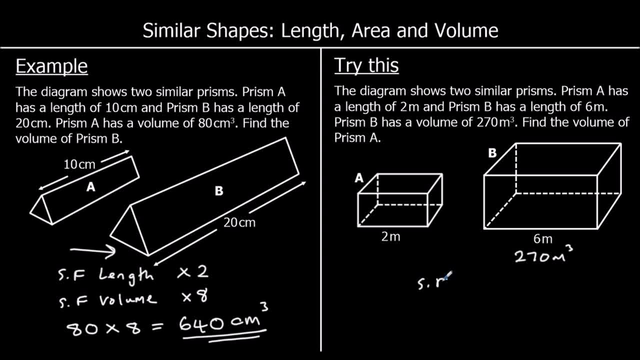 prism A. So the scale factor for length, What do I do to get from 2 to 6?? So 6 divided by 2 times by 3.. Scale factor for volume is scale factor cubed. So 3 cubed is 27.. 3 times, 3 times 3.. 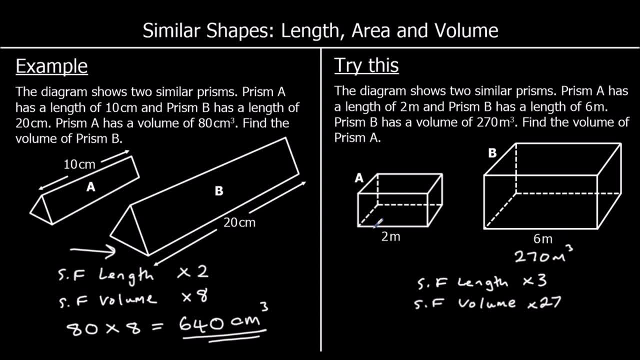 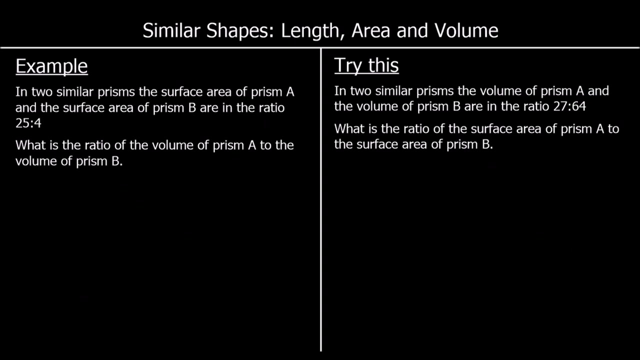 So, to go from the big shape to the little shape, we're going to divide by the scale factor. So it's going to be 270 divided by 27,, which is 10.. So it's 10 metres cubed. Okay, a different type of question. So in two similar prisms, the surface area of prism A. 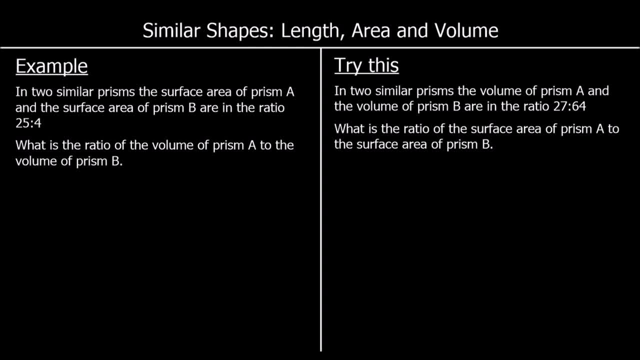 and the surface area of prism B are in the ratio 25 to 4.. What's the ratio of the volume of prism A to the volume of prism B? So the ratio of prism A to the volume of prism B is 25 to 4.. 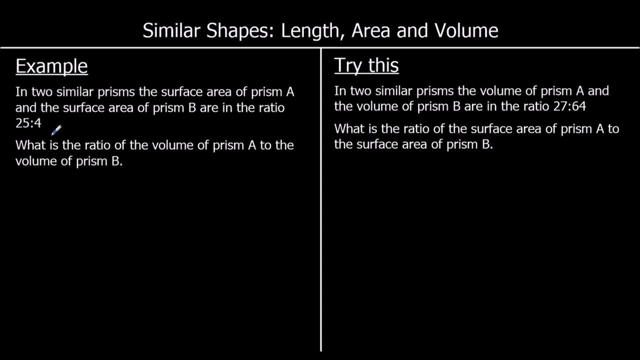 So this is the scale factor for surface areas. So area scale factor is scale factor squared. So for area we have 25 to 4.. If we want to find the scale factor for length, we've got scale factor squared at the moment. 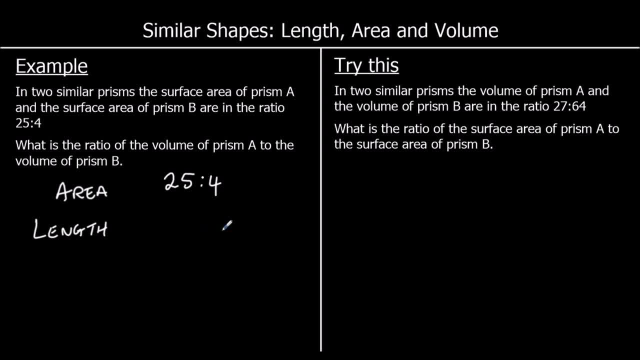 So to find scale factor, we square root. So if we want to find the scale factor for length, we square root. So for length, the scale factor will be square root 25 to square root 4,, so 5 to 2.. 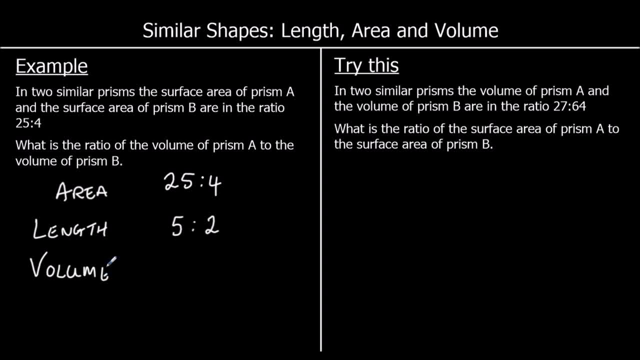 So the scale factor for volume is scale factor cubed. So we're going to take our length scale factor and cube it. So 5 cubed 5 times 5 times 5 is 125, and 2 cubed is 8.. 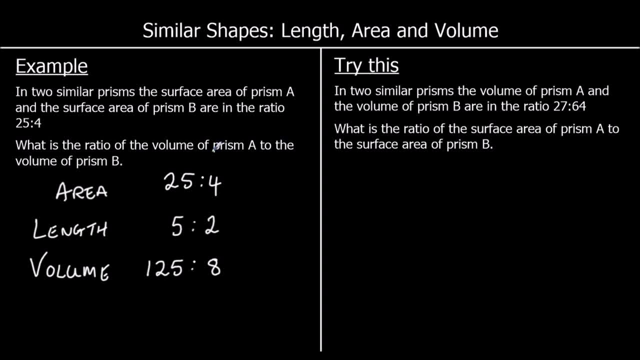 So the ratio of the volume of prism A to the volume of prism B is 125 to 8.. OK, one for you to try, So pause the video, give it a go This time. in two similar prisms. the volume of A to the volume of B is, in the ratio, 27 to 64.. 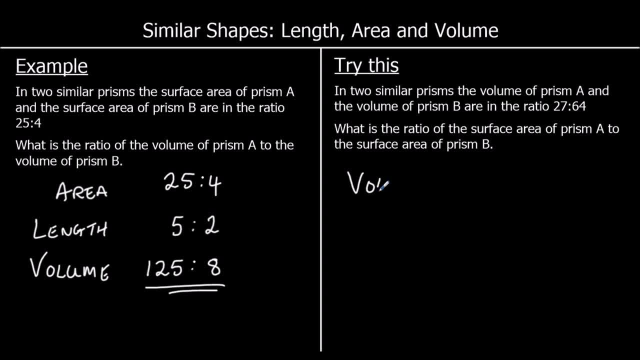 So this is volume this time And we want to work out the ratio of area. So scale factor for volume is scale factor cubed. So to find the scale factor for length we're going to cube root. So the cube root of 27 is 3, and the cube root of 64 is 4.. 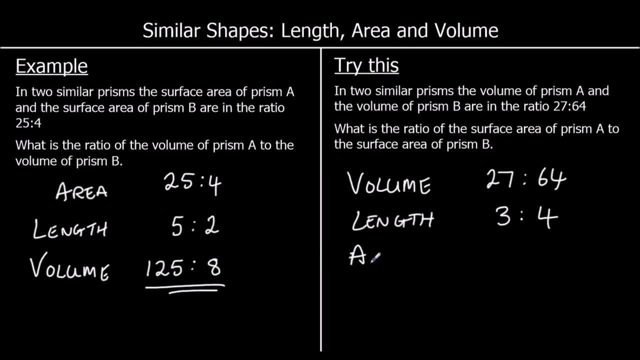 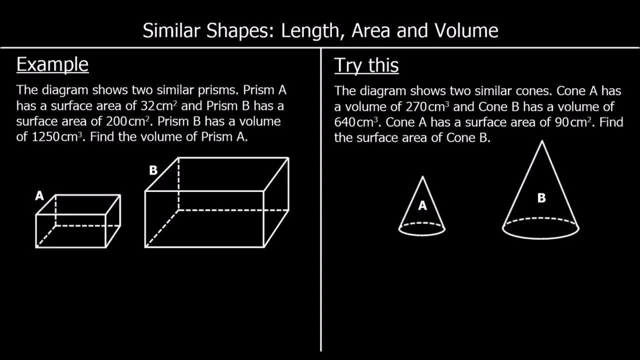 OK, OK. And then to find the scale factor for area, we're going to square the scale factor, So 3 squared is 9,, 4 squared is 16.. And one more example. So this time we've got two similar prisms again. 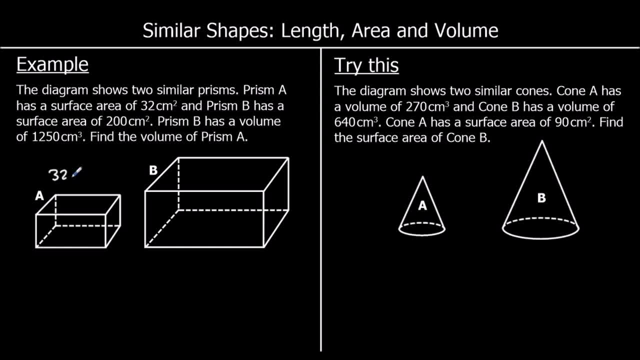 Prism A has a surface area of 32 centimetres squared. Prism B has a surface area of 200.. And we're given prism B's volume of 1,250 centimetres cubed And we need to find the volume of prism A. 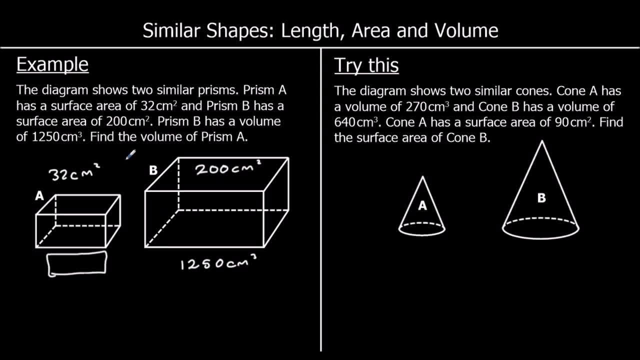 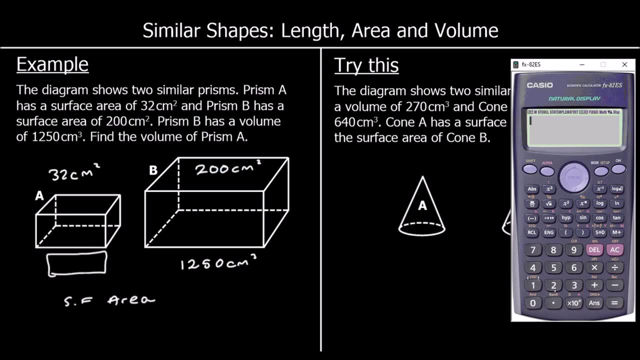 So let's look at the scale factor for areas And we can work that out. So scale factor for area. So what do we multiply 32 by to get 200? So if we grab a calculator and do 200 divided by 32,, 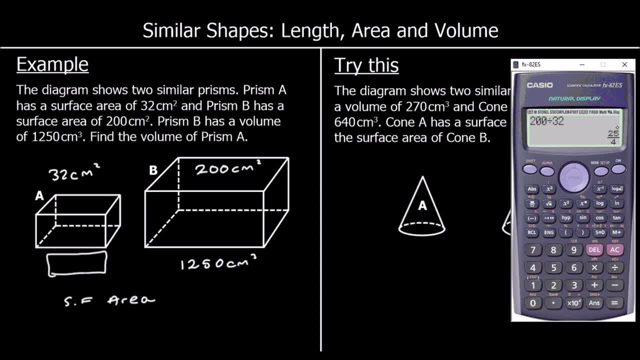 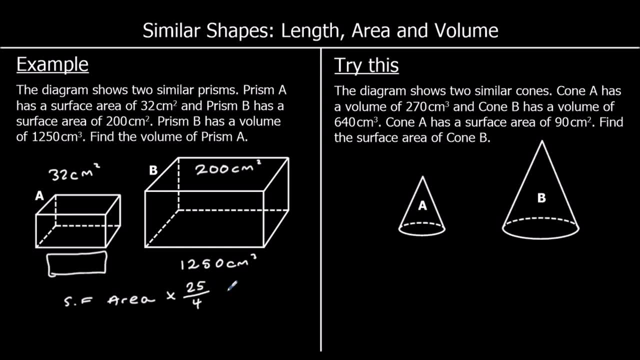 that's 25 over 4.. And I'll leave it as a fraction. So times 25 over 4.. So that's our scale factor for area. If I want scale factor for length, I'm going to square root. So if I square root 25 over 4,. 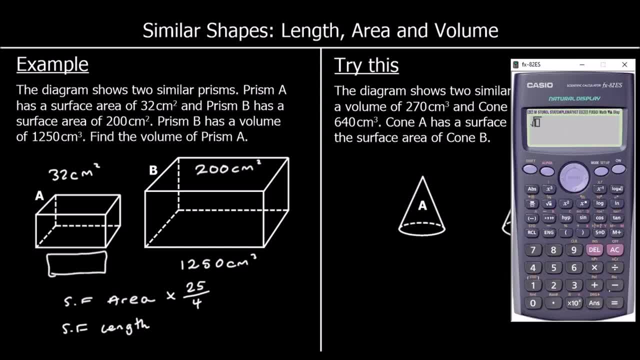 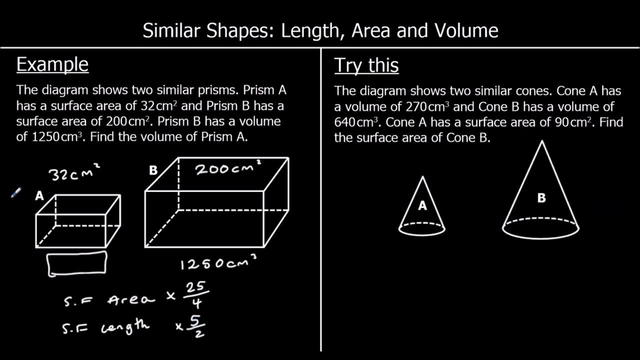 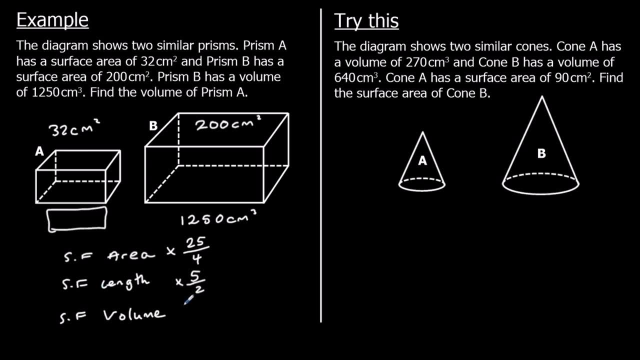 I don't have to use a calculator, I will. So square root the answer, That's 5 over 2.. The scale factor for length is 5 over 2.. And to get scale factor for volume, that's scale factor for length cubed. 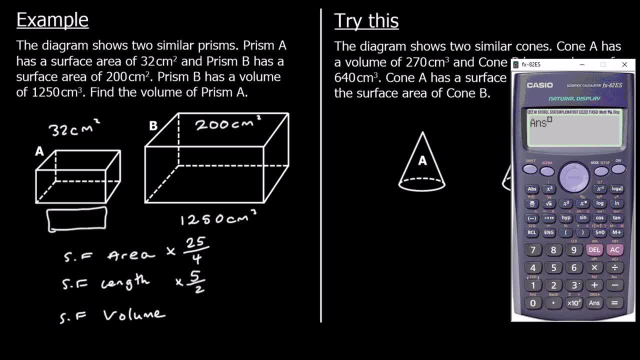 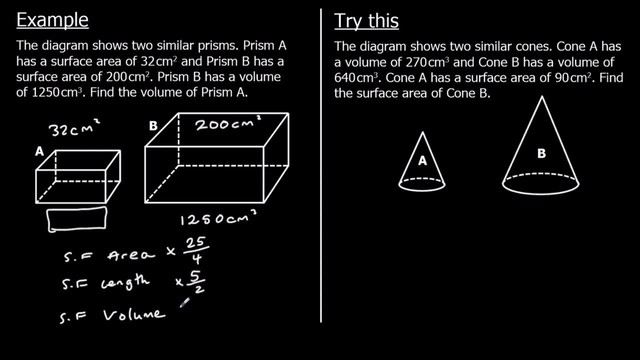 So this answer cubed and that's 125 over 8.. So our scale factor for volume is times 125 over 8.. So to go from little shape to big shape, we times by 125 over 8.. To go from big shape back to little shape: 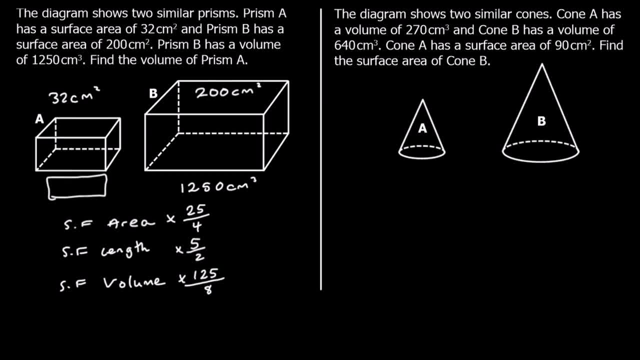 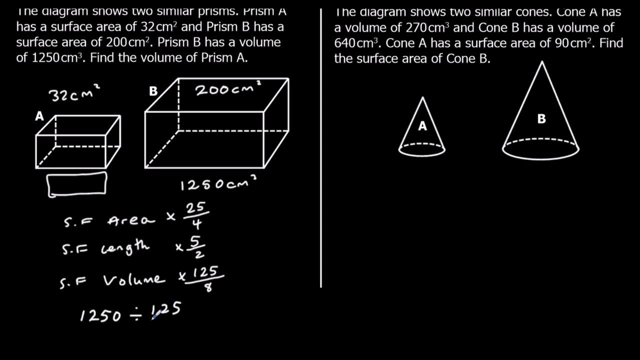 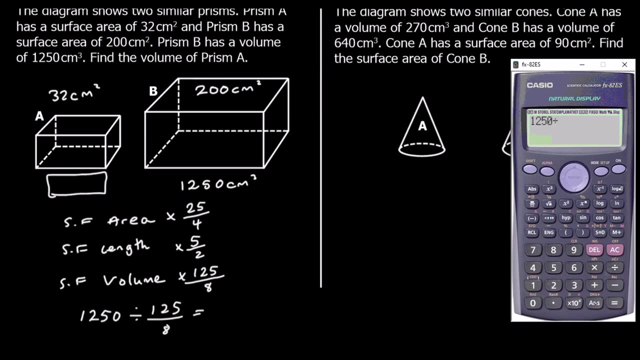 we will divide by 125 over 8.. So we're going to get 1250, divided by our scale factor for volume, And that will tell us the volume of the smaller shape, Which is 80.. So that's 80 centimetres cubed. 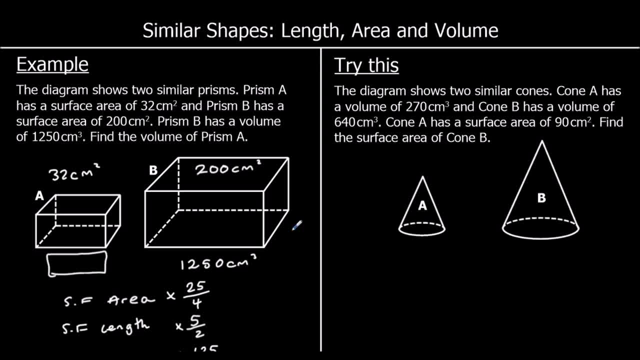 Okay, one for you to try. So pause the video and give it a go. So we've got two similar cones. We've got volume of cone A, 270 centimetres cubed, And the volume of cone B Is 640 centimetres cubed. 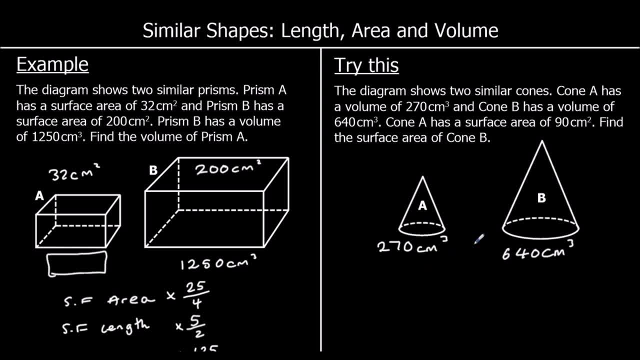 So we can work out the scale factor for volume. And if we do 640 divided by 270, we will get scale factor for volume, And I'm just going to write that as 64 over 27.. So that's our scale factor for volume. 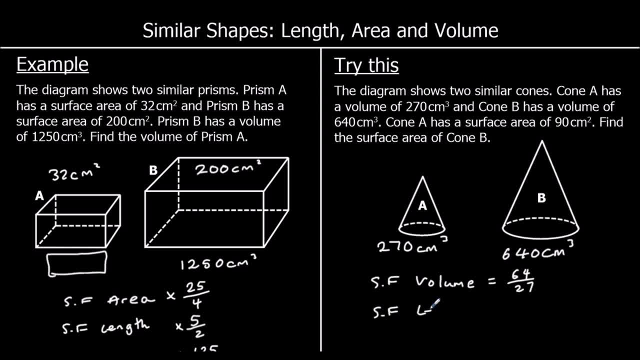 To find the scale factor for length, we are going to cube root. So volume scale factor is scale factor cubed. So if we cube root this, which is 4 over 3, we get our scale factor for length And we want to work with surface area. 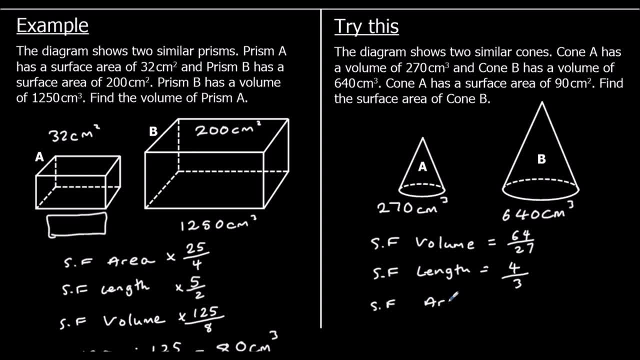 So we're going to square the scale factor 4 over 3. times 4 over 3 is 16 over 9.. So our scale factor is times 16 over 9 to go from little to big. And that's what we want to do. 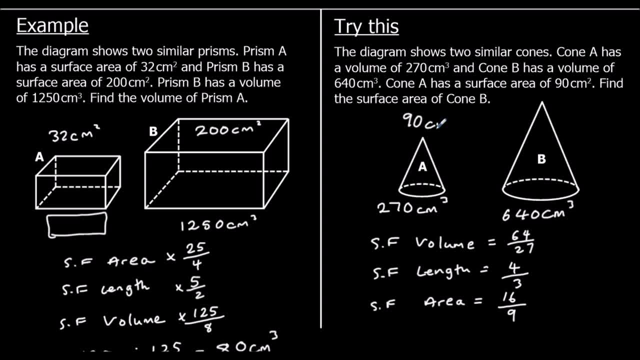 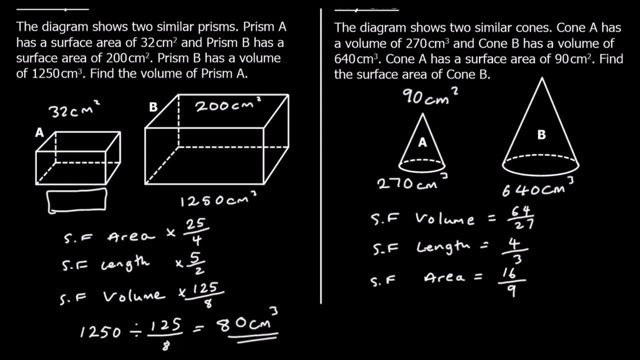 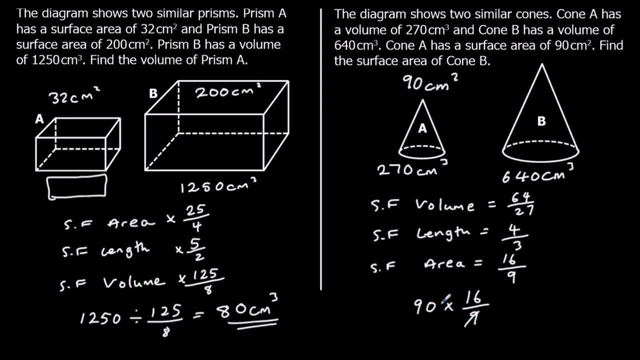 So cone A is a surface area of 90 centimetres squared. So we're going to do 90 centimetres squared times the scale factor. So 90 times 16 over 9.. So we can say that's 10 times 16.. 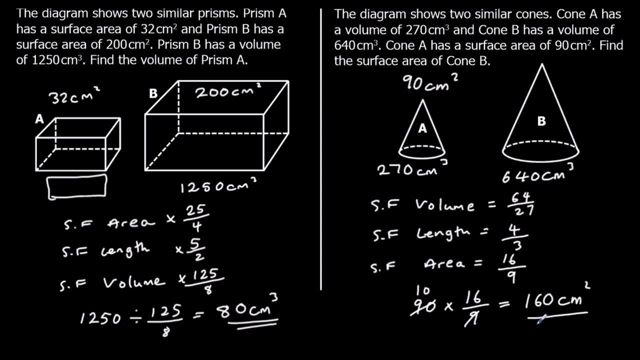 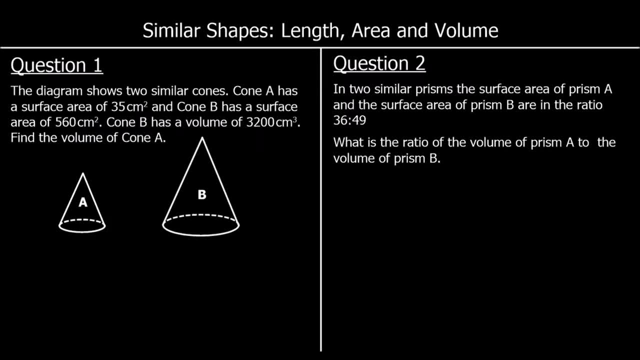 Which is 160 centimetres squared. OK, two questions to finish up, So pause the video and give them a go. Question one says: the diagram shows two similar cones. Cone A has a surface area of 35 centimetres squared. 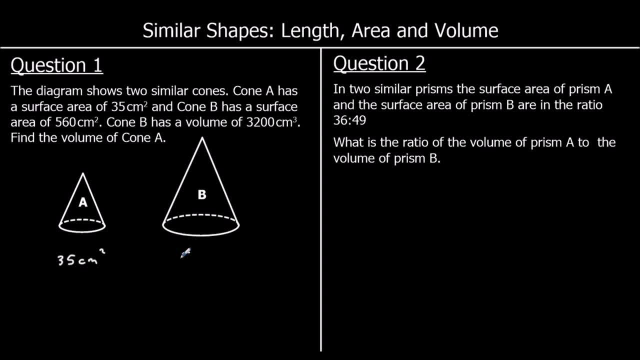 And cone B has a surface area of 560 centimetres squared And cone B's volume is 3,200 centimetres cubed And we need to find cone A's volume. So let's work out the scale factor for areas. 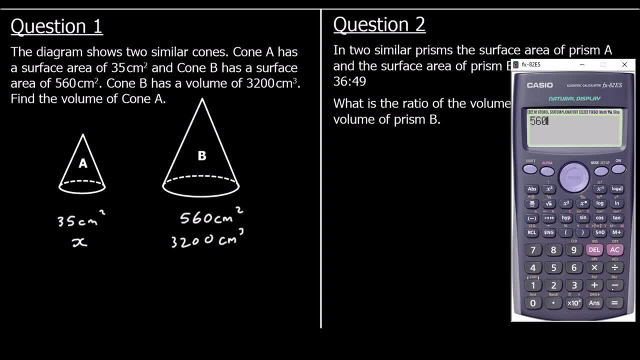 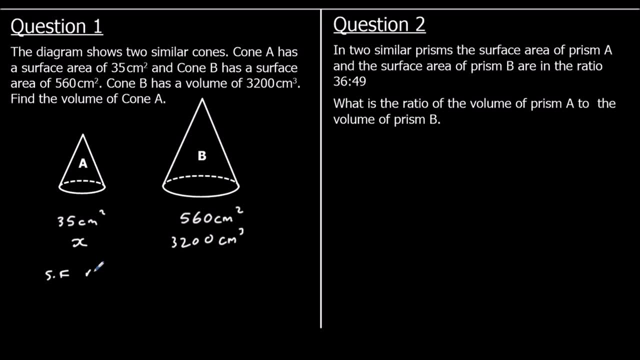 So if I do 560 divided by 35, which is 16.. So the scale factor for area is times 16.. The scale factor for length is going to be the square root of that. So scale factor for area is scale factor squared.